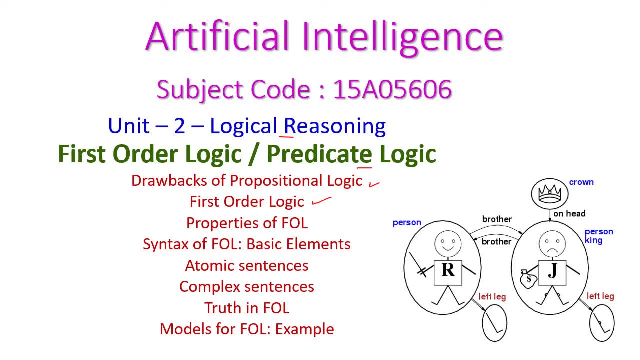 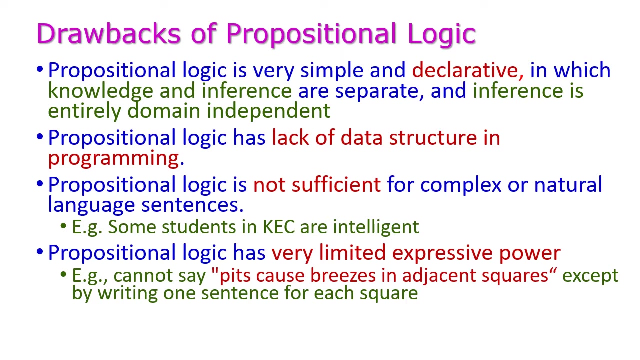 After that, the definition of first order logic, properties of first order logic and the basic symbols or basic elements of the first order logic, atomic and complex sentences, truth in first order logic and a model for first order logic. We will see one example for this also. First, let us see the drawback of propositional logic, because on the base of propositional logic the first order logic being developed. 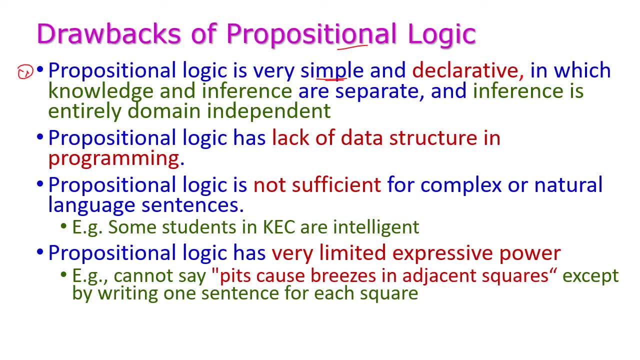 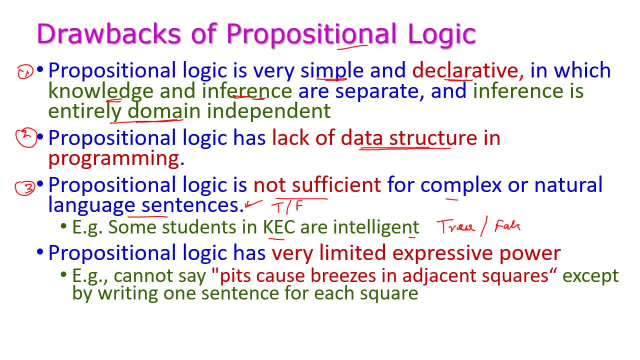 And the third one is: propositional logic has lack of data structure in propositional logic. Now you can notice that auko, meaning false, will also come here. hence these types of statements can not be accepted by this propositional logic. And the forth drawback is: propositional logic has very limited x-perhesive power. 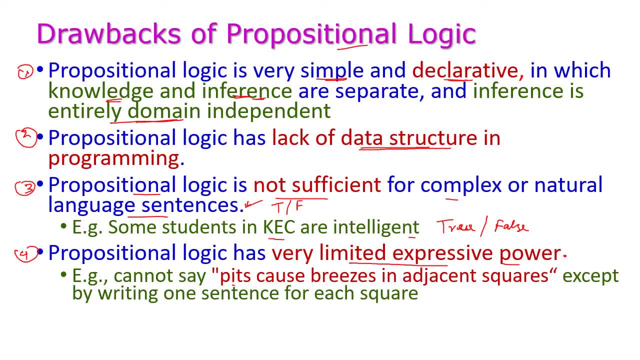 For example, we cannot say PITs causes breeze in adjacent square in the Wampus world, OK, If there is a pit in one square, the adjacent squares will get breeze. So if it is pit means these are all breeze, Isn't it? 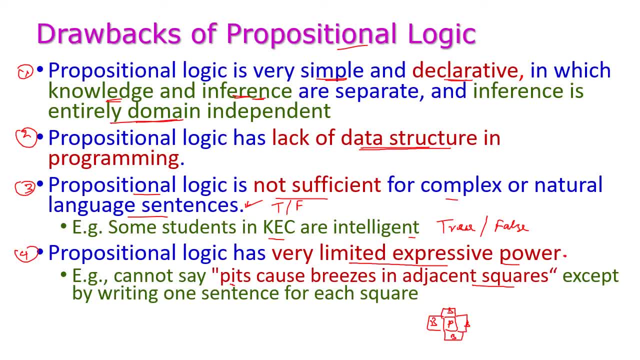 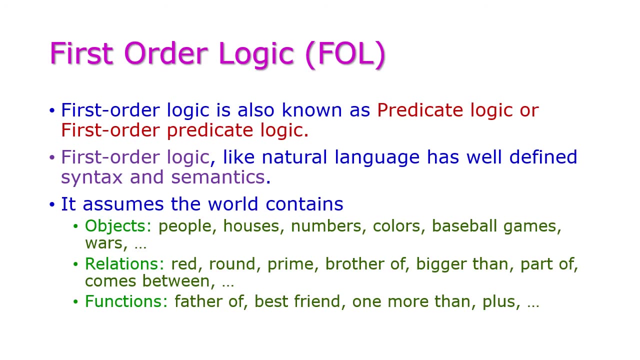 But we cannot express all these things in one sentences, Because the propositional logic will accept one sentences for each square. For each square we have to write separate sentences. Okay, this is another drawback in propositional logic. So to overcome the propositional logic, here we introduce the first order logic. 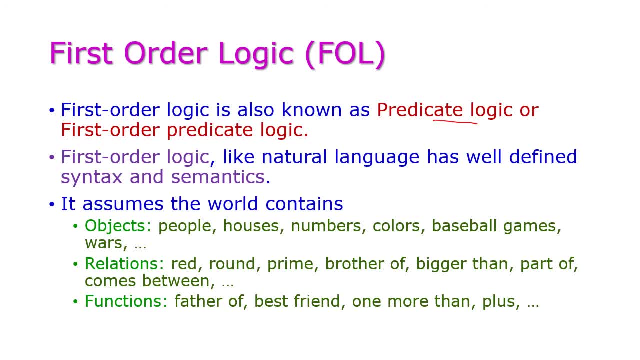 The first order logic is also known as predicate logic or first order predicate logic. It is simply called as FOL. FOL means first order logic. Here, the first order logic is like a natural language, as well as defined syntax and semantics. That is, the FOL is having. 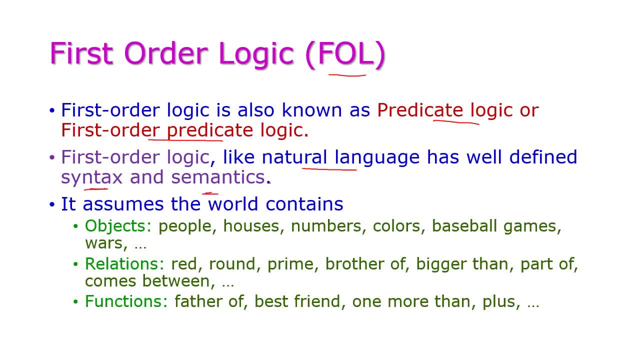 A very powerful syntax and semantics And in FOL it assumes the world contains World means agent world, Agent world or agent environment contains objects, relations and functions. Okay, it contains, That is the world contains all objects, the relation between the objects and the functions of objects. 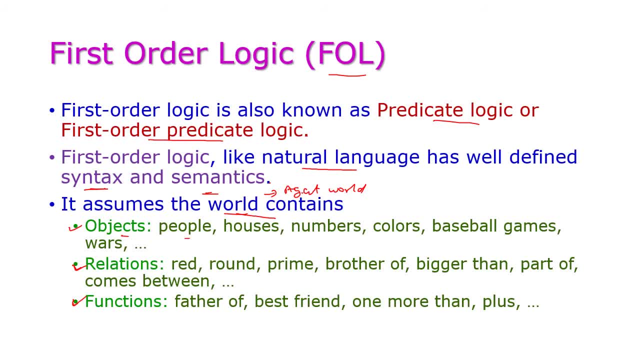 Otherwise okay Objects. example: people, houses, members, colors, baseball game, VAS and etc. These are all objects. Any real world entity is called as object Right And next one is relation. Relation means the unary relation between the object. 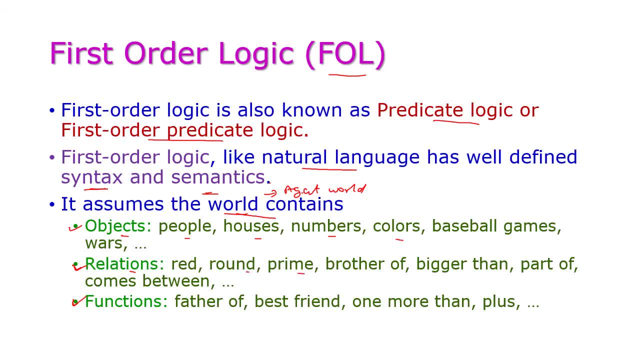 Okay, Red round, prime brother of. bigger than part of. comes between and, etc. Okay, less than greater than. These are all relations And functions: father of some x. best friend of one or more than square root. add, multiply. 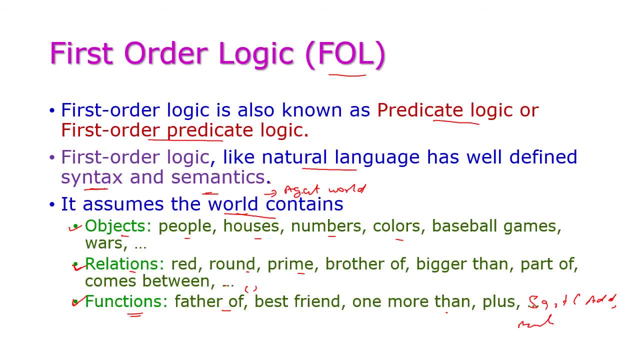 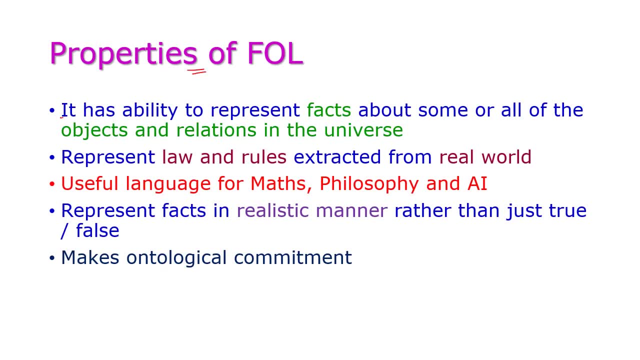 Okay, So these are all functions, And next let us see the properties of first order logic. Here the first order logic has the ability to represent the fact about, Some are all of the object and their relationship with the in the universe. 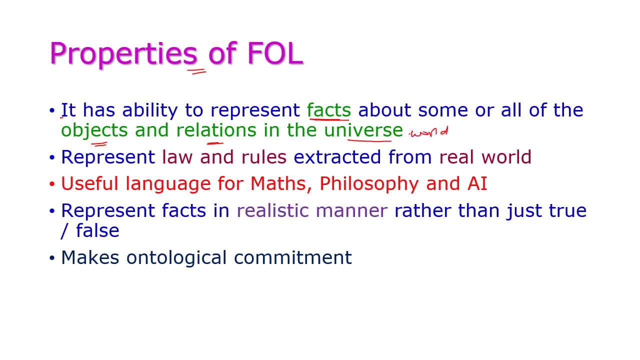 Universe means world, Agent world. Okay, So by using first order logic we can represent almost all the facts about all the objects and relation and functionalities of object, everything Here. it represent laws and rules Extracted from the real world and the useful that is. it is useful for representing mathematics. 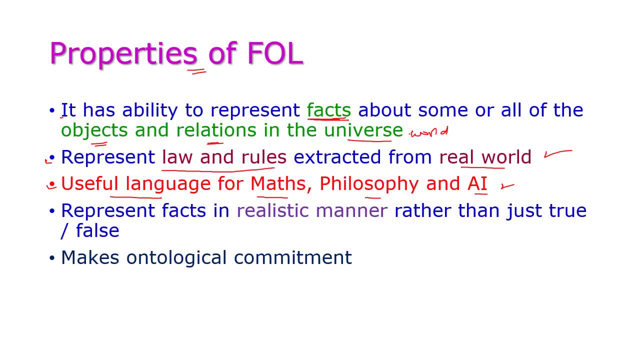 philosophy and artificial intelligence also. And the first order, logic, represent fact in realistic manner rather than just true or false Like the propositional logic. Okay, Here we can represent in realistic manner. Okay, Here we can represent in natural manner, like the natural language. and it makes ontological. 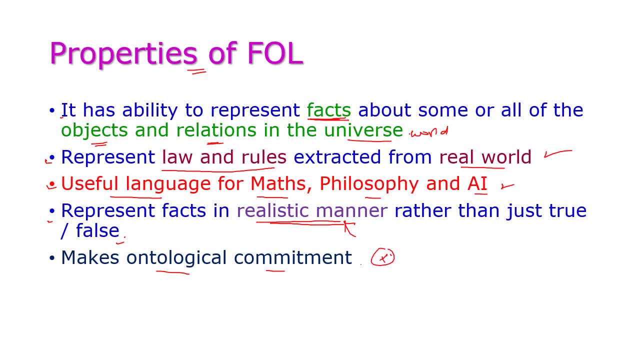 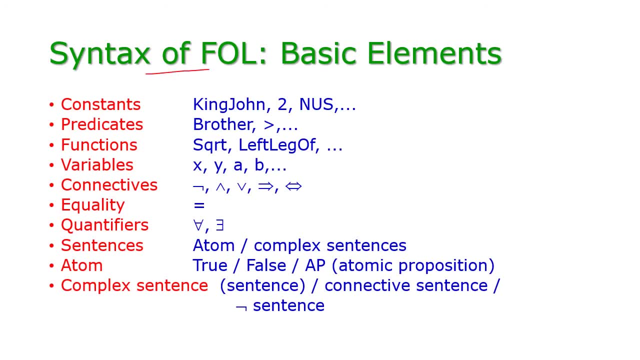 commitment. This is most important property of first order logic. And next let us see the syntax of first order logic. That is, the basic elements that will come for syntax in first order logic. The first one is constant, Constant. Okay, 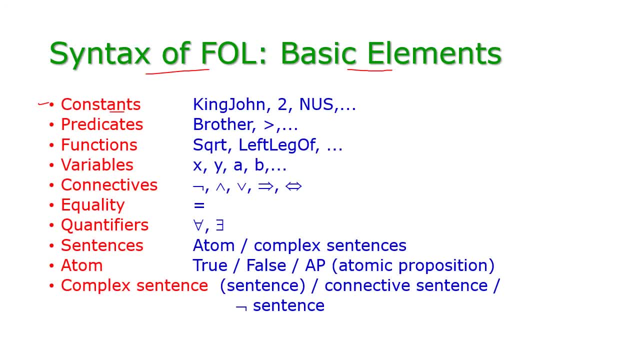 All the nouns, numbers, places will come under constant. King John, number two: NUS, KES. Okay, So all these things will come under constant And predicate Here, brother, greater than, less than, less than or equal to. 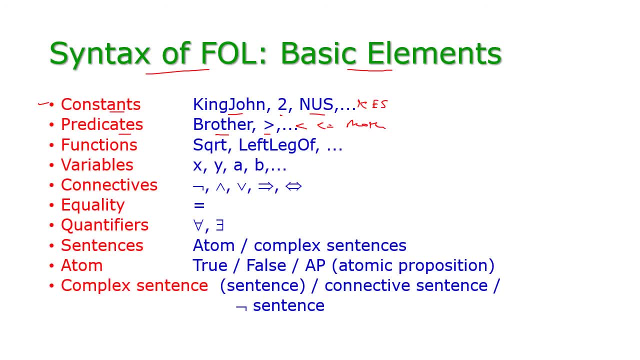 Okay, Mother, Everything will come under predicate. And next one is function Function here, square root, left leg of father of. Okay, All the things are under constant. And next one is function Function here, square root, left leg of father of. 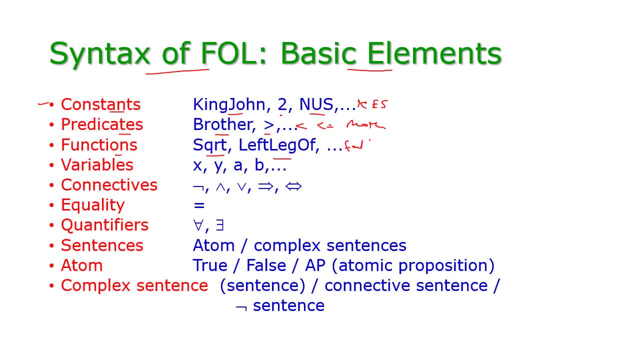 Okay. And the following is the function. The first one is the function Father of Okay. so these are all functions: Square root, add, multiply, Okay. and next one is variables. Here we have to use the small letters of English alphabet to represent the variables and connectives. 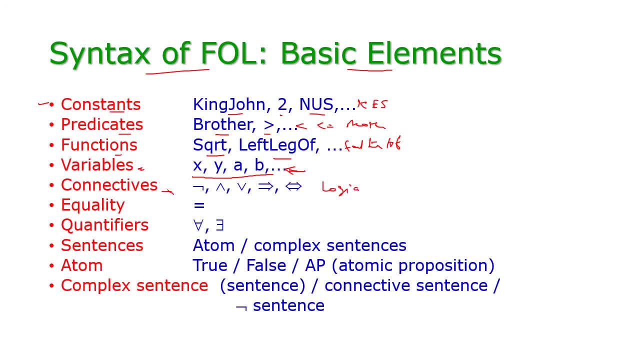 So these are all logical connectives. Okay, we are having five logical connectives: Negation, conjunction, disjunction, implication and biconditional. Okay, so these are all the different connectives which are used in first order: logic. 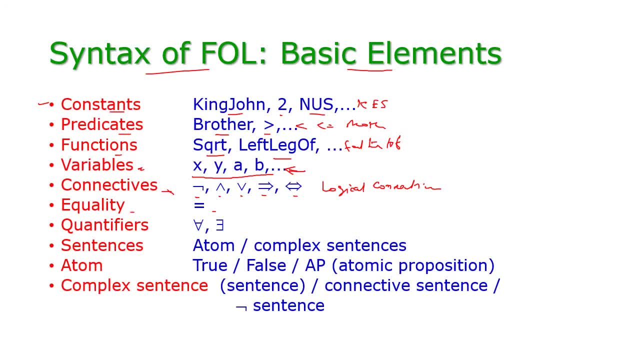 And next one is equality. That is, equal symbol. This is used to represent the two terms are equal. and next one is quantifiers. this is very important here. okay, so two quantifiers are here. this is for all, and this is. there exist universal quantifier and existential quantifier. and next one is: 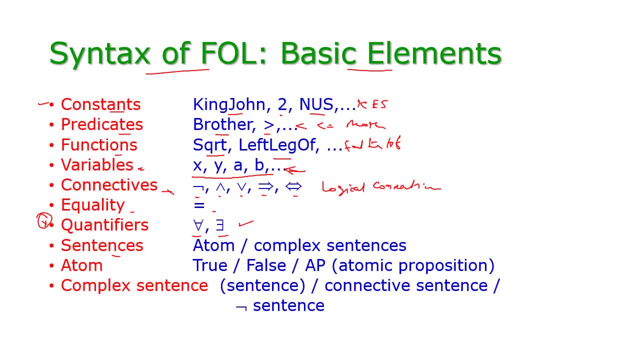 sentences. here we are using two types of sentences, that is, atomic sentences and complex sentences. atomic sentences and complex sentences. what is atomic sentences? it contains either true or false, or atomic propositions. atomic propositions: any simple sentence, whatever it may be. and what about the complex sentences? the sentences within this bracket, connective sentences by. 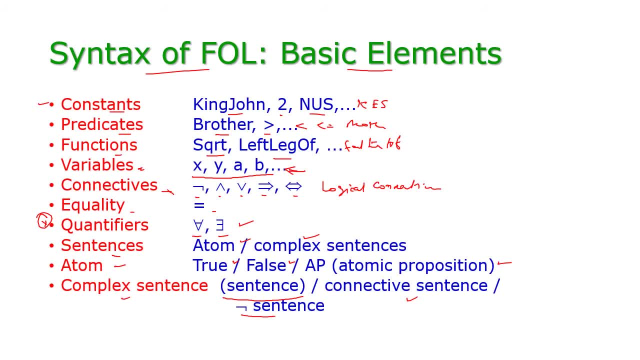 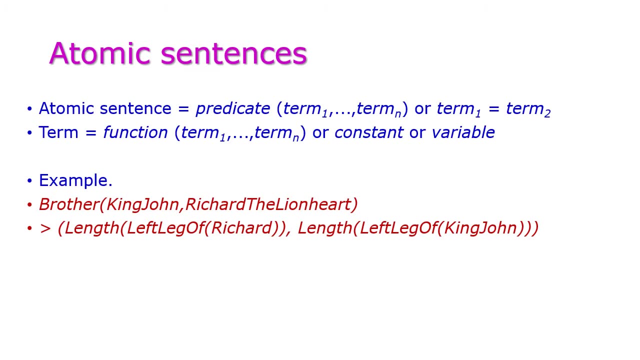 using the logical connectives or negative sentence. okay, so the complex sentences will be constructed- atomic sentences- with the logical connectives. first let us see the atomic sentences here. the syntax for atomic sentences is: atomic sentence equal to predicate of term 1 comma, term 2 comma, term 3, etc. up to term n or term 1 is equal to. 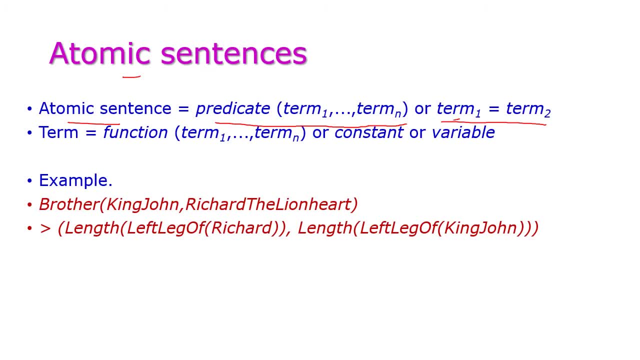 term 2. and what is the term here? term may be the function of term 1 comma, term 2 comma, term 3, etc. up to term n, or the term may be a, or the term may be a variable, a single variable. okay, so this is the syntax for atomic sentences. 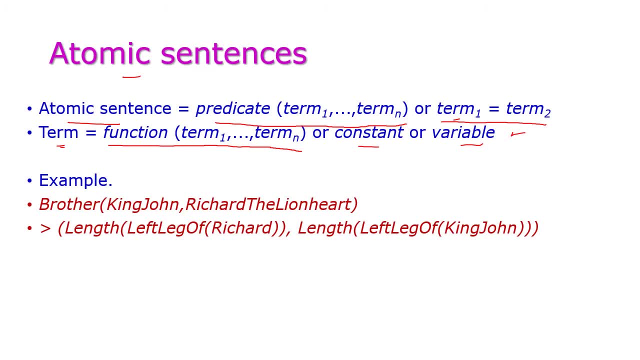 let us see one example for this here. the first one is brother of king john comma, richard the leinhardt. that is, king john and richard the leinhardt are brothers. brother is a relation here. that is the predicate. and next one is the length. that is greater than, greater than. 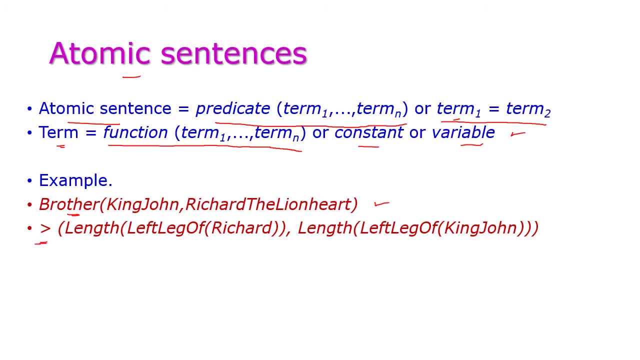 length of left leg of richard. comma length of left leg of king john, that is, the left leg of richard, is greater than the length of left leg of king john. okay, so the king- sorry, the richard's left leg of king john is greater than the length of left leg of king john. 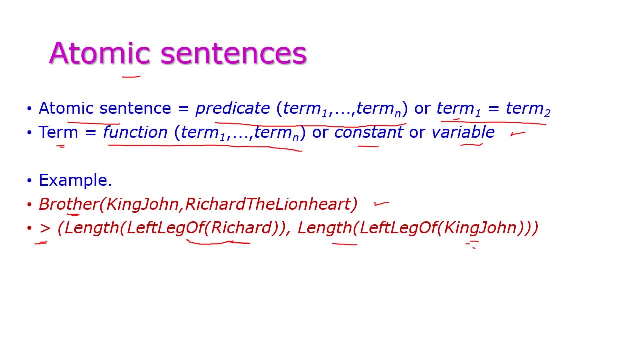 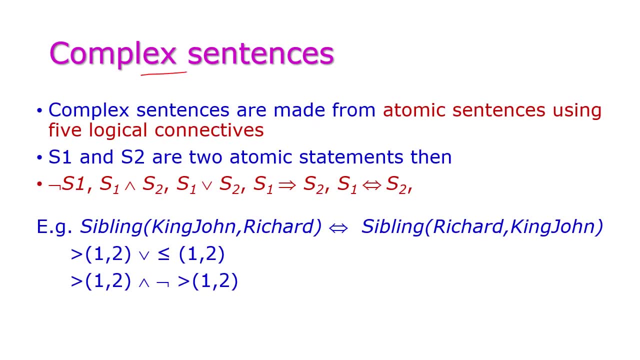 is greater than king john's left leg. so this is the example for atomic sentences. and next let us see the complex sentences. the complex sentences are made from atomic sentences by using five logical connectives. okay, for example, suppose s1 and s2 are two atomic sentences. 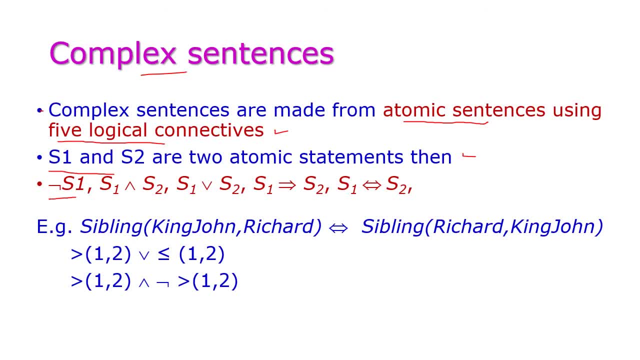 then we can construct: not s1- that is negation of s1- are not s1, that is negation of s1- are s1 and s2? this is the conjunction s1 or s2, this is disjunction s1 implies s2. implication s1: biconditional s2. if and only if. this is if, then, and this is if and only. okay, by using all. 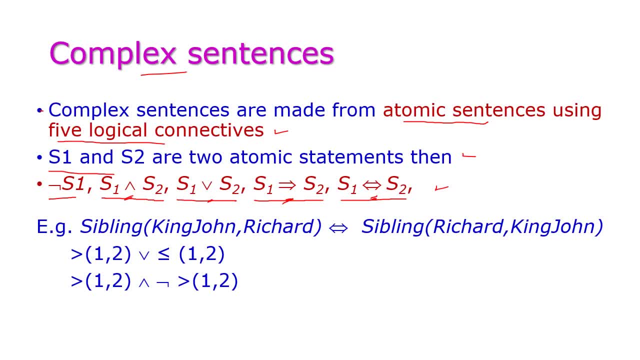 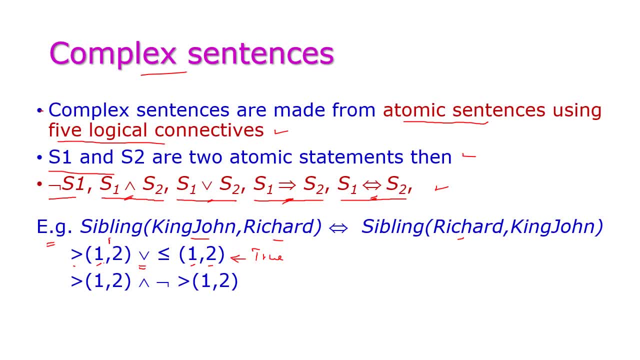 1 is greater than 2. this will give false value. r- this is r. 1 is less than or equal to 2. this will give true value, isn't it? so the result will be true. and next: ok, greater than or of 1 comma 2 and not greater than of 1 comma 2. ok, so this is false and the entire thing will be. the entire thing will be true, but 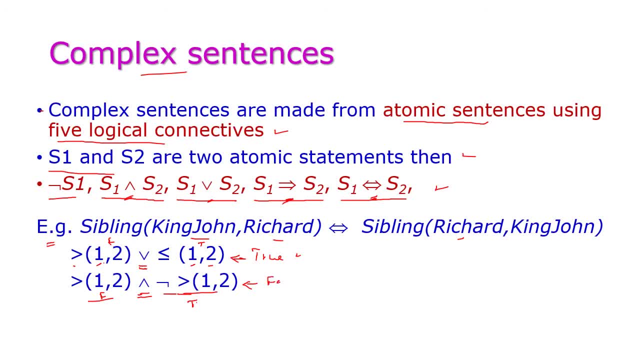 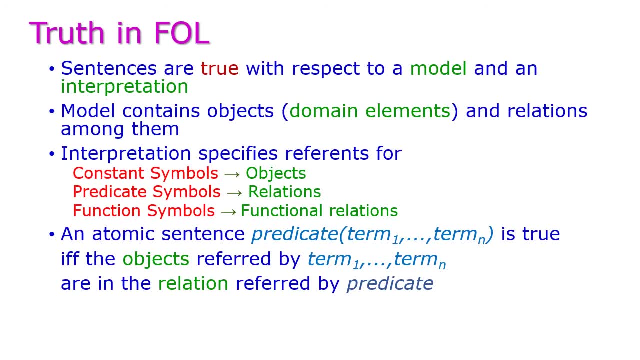 here. this is conjunction, so the result is false. ok, so this is the example for complex sentences, and next we will go to the truth of first order logic here. a sentence in first order logic is true with respect to the model and the interpretation, so based on the model. 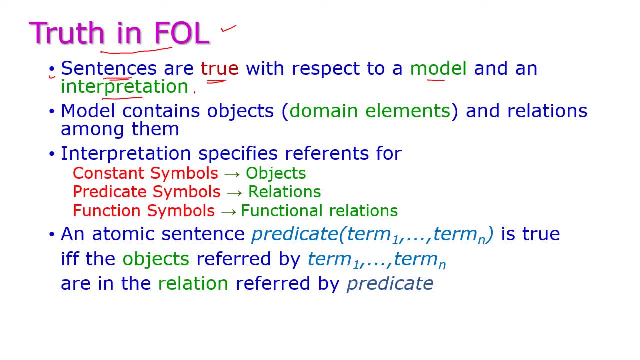 and interpretation. only. we can consider a particular sentence, ok, and the truth value of that sentence will also respect to the model here. model contains objects. model contains objects, relations and functions. relations and functions: ok, objects means any domain element. any domain element is called as object. so this is called as model. and what is? 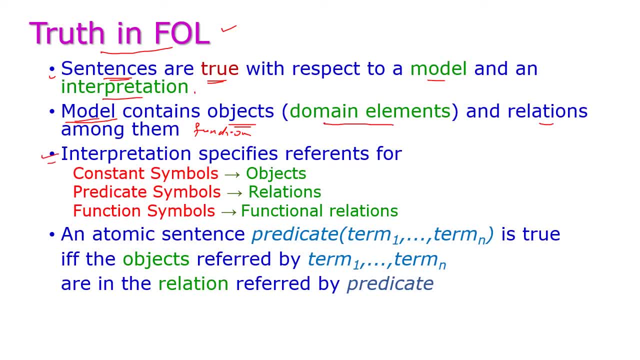 interpretation here, that will be the interpretation of the szczególities. we will see that when a text is a variable, when a text is a constant largest, and when a text is a vertex and a vector, when a text is a quarter value, when text field is a subscript function, 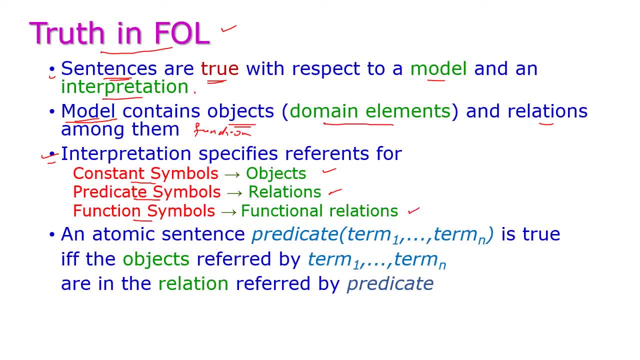 when it is a clerical object and then a socialA variable when a child enters the好了. when is a total value of now? so first let us see this, the first part. what is this? is a practice up to term n, which is true, which is true if and only if, objects referred by term 1, etc. up to 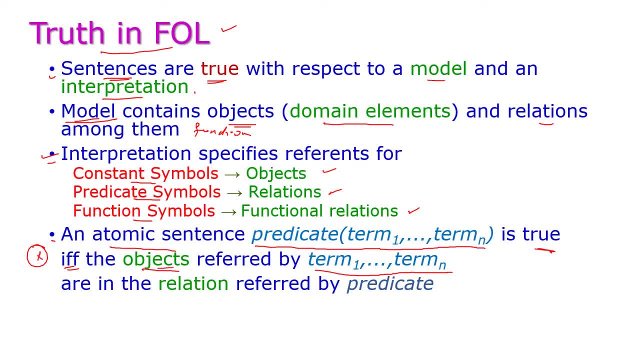 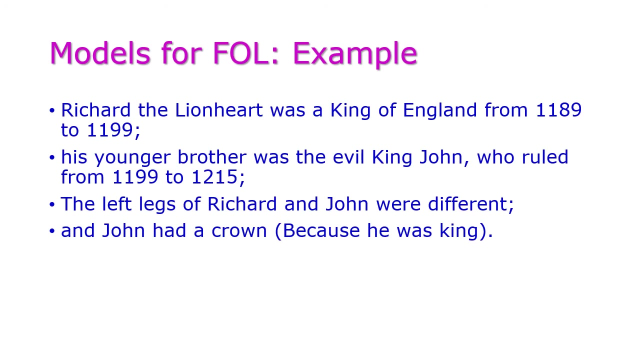 term n. all the terms should represent these objects are in the relation which is referred by the predicates. okay, otherwise the sentence will not accepted by this first order logic. okay, so this is very important. here and now we will see one example for this first order logic here. the Richard the Lionheart was king of England from 1189 to 1199, and his younger 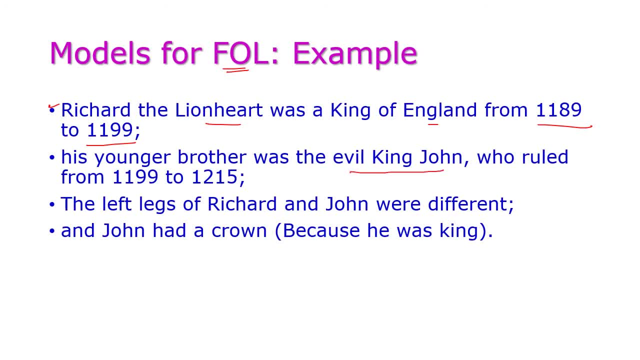 brother was evil King John, who ruled from 1199 to 1250, and the left leg of Richard and his left leg of Richard and his left leg of Richard and his left leg of Richard, and. and his left leg of Richard and his left leg of Richard and his left leg of Richard, and. 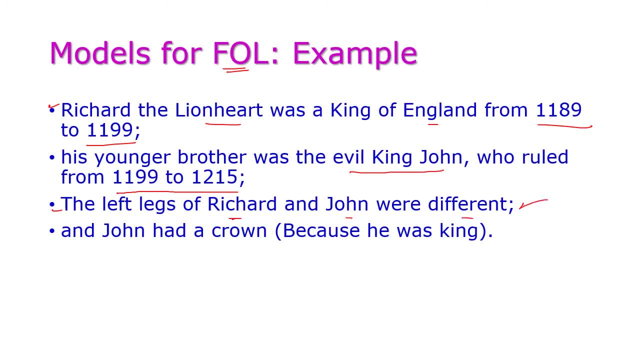 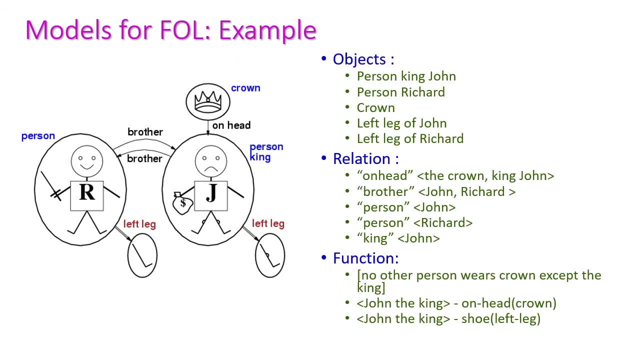 John were different. okay, because the Richard left leg is lengthier than John's left leg and John wore shoes because he is king. after that, John had a crown because John was king. see, for this, we will draw this diagram. okay, so this is Richard the Lionheart and this is 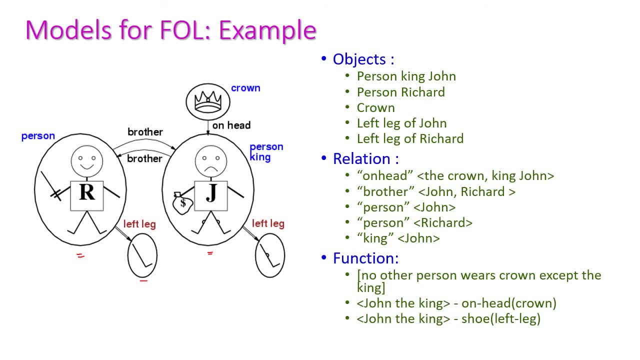 King John. okay, and this, this is left leg, left leg of Richard the Lionheart and King John are different and crown, crown, because the John is king, so he is carving crown. okay, so from this diagram we are going to extract the objects. what are the possible objects here? 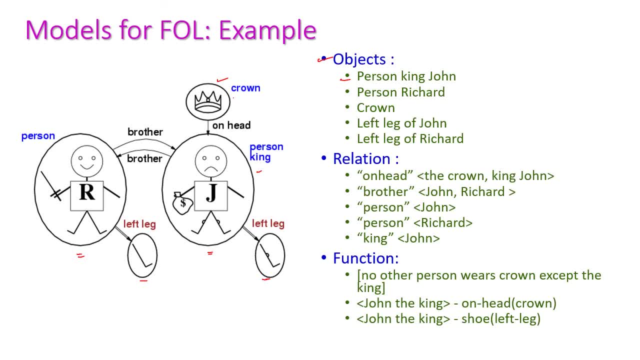 person. King John is a person, okay, and Richard is also a person. crown is there, this is also an object and left leg of John, left leg of Richard. so there are totally five objects and the relations. what is the relation here? on head, the crown comma, king john. so crown is on the person. 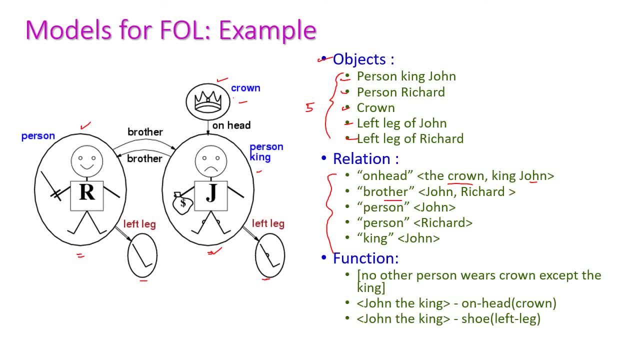 king john, okay. and next one is brother relation. john and richard are brothers. and next one is person: john is a person, richard is also person. king is also relation. king of john, okay. so totally, five relations are there and next the functions. okay, here no other person wears crown except the. 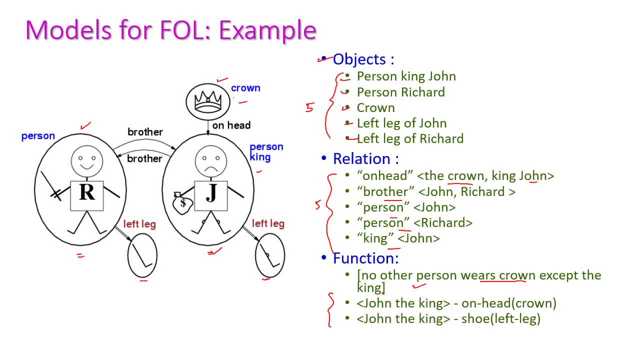 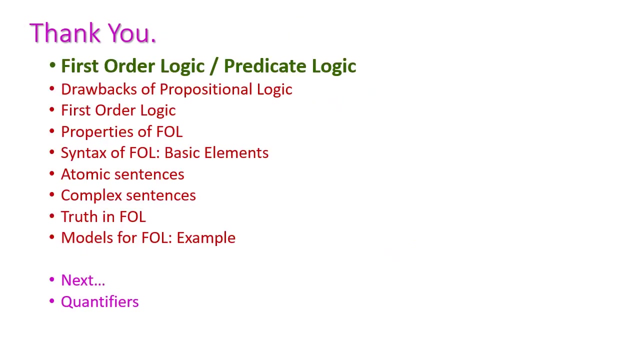 king, except the king. okay, so john the king on head crown. okay, so king is having crown on his head and king wears shoe on his left leg. okay, so these are the functions. up to this. we have seen the introduction about the first order logic, which is otherwise called. 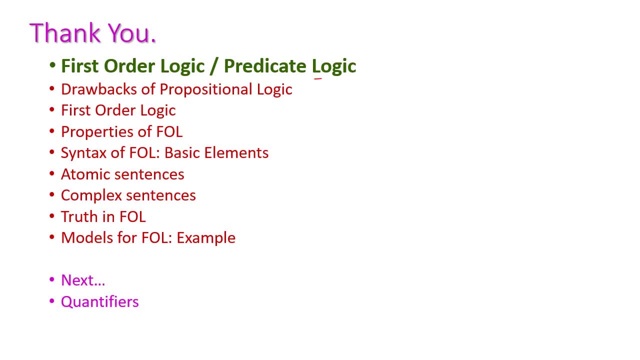 as predicate logic. under this lesson we have seen the drawbacks of propositional logic and the definition of first order logic, properties of first order logic and the basic elements of first order logic: atomic sentences and complex sentences, truth in first order logic- and we have seen one example also. 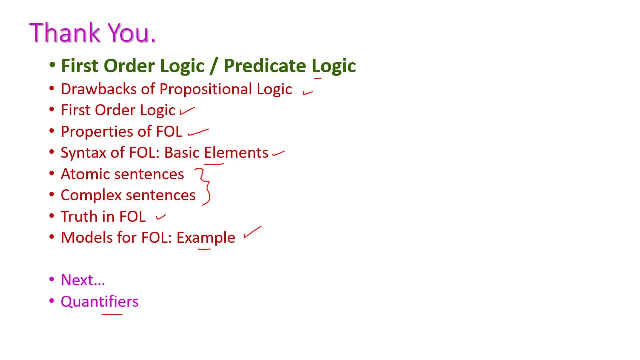 in this video we have seen two basic elements of first order logic. In the next class we will see the quantifiers. Two quantifiers are there for all and there exist. Okay, if you have any doubt, you please give in the comment box. Thank you.